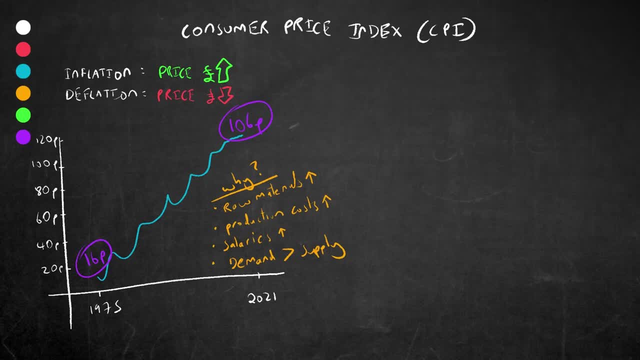 inflation and, as such, have developed ways to do this. so let's talk about cpi, one of the common measures. cpi is a theoretical basket of everyday goods, each with an average price tag. now there are hundreds of everyday goods and services that are tracked, and they are split into eight categories. 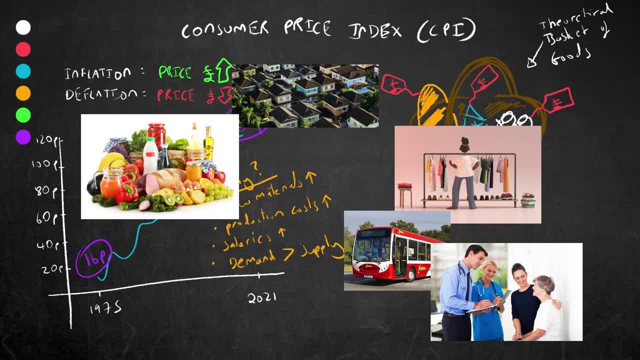 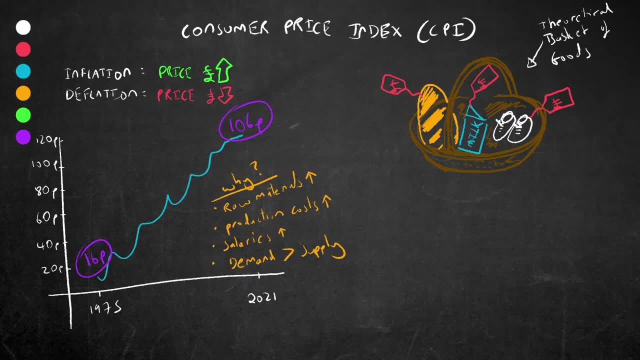 namely housing, clothing, transport, food and drink, medical care, recreation, education and other. examples within these categories might include the price of a carton of milk, a loaf of bread, rent, a pair of shoes, electricity and so on. these also depend what country you are from the basket of. 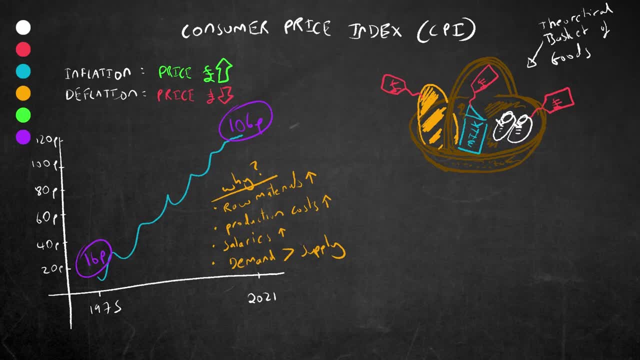 goods in the uk will be different from the basket of goods in the us, and this basket is also dependent on the times of which we live. for example, in 2020, hand sanitizer was added to this list. cpi is always measured against a base year, so if the average cost of a basket in 2021 is 5 pound 20 and 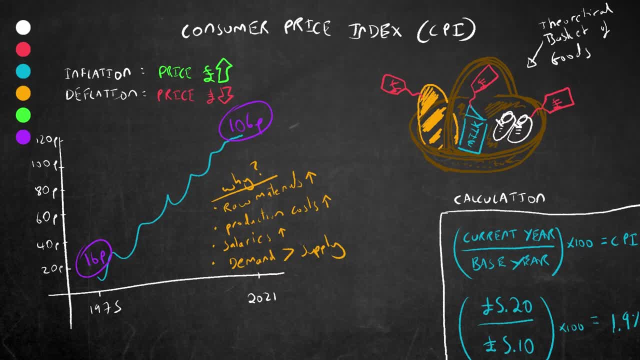 the average cost of that same basket in 2020 is 5 pound 10. the increase is 5 pound 20 divided by 5 pound 10 times 100, which is 1.019, or simply 1.9 percent rise. cpi helps determine the purchasing. 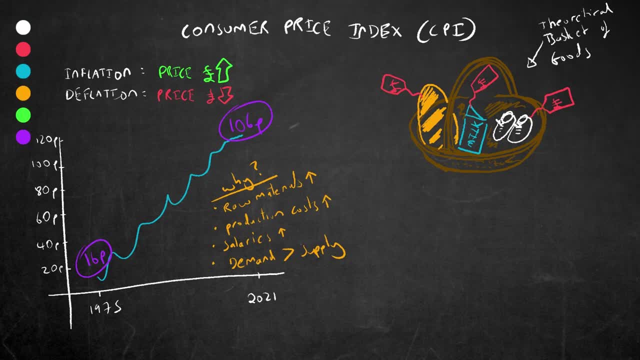 power of a currency and consequently the rate of inflation. the government here in the uk aims to keep inflation at the two percent level. the general view of the market is that the market is. the general view is that if inflation is too high or changes a lot, it's hard for businesses to set. 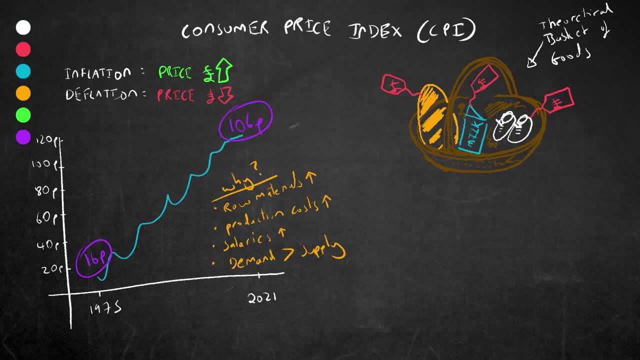 the right prices for their products and for people to plan their spending. on the other hand, if it is too low, then people might not spend as much as they expect prices to fall, which stops the economy from growing. having said that, the reason why everyone is talking about it now is that inflation in the 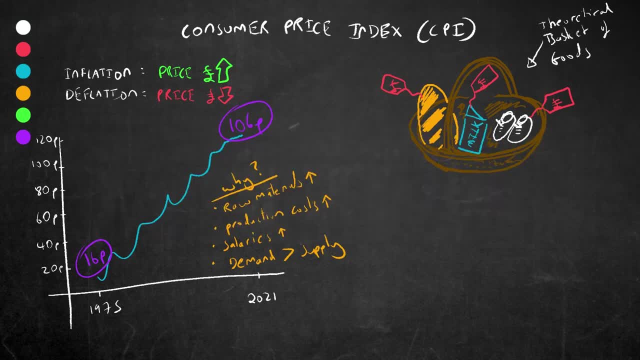 uk is now as high as 5.1 percent. now, when we talk in terms of loads of bread, it's hard to see how a five percent rise in prices is impactful in the everyday. however, it really is and it's something to take seriously. let's take a broad example. say: in 2021, you receive a net salary of 30 000 pounds. 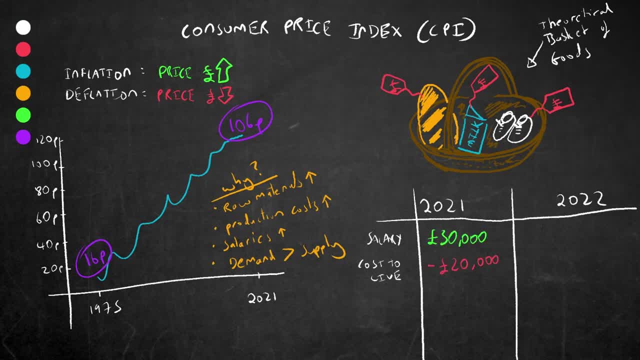 a year and your cost of living bills, rent car etc. comes to around 20 000 pounds a year, so you manage to put 10 000 pounds away in savings. on a five percent inflation rate, your cost of living in one year's time, in 2022, will essentially be 21 000 pounds now, if your salary doesn't go up accordingly.